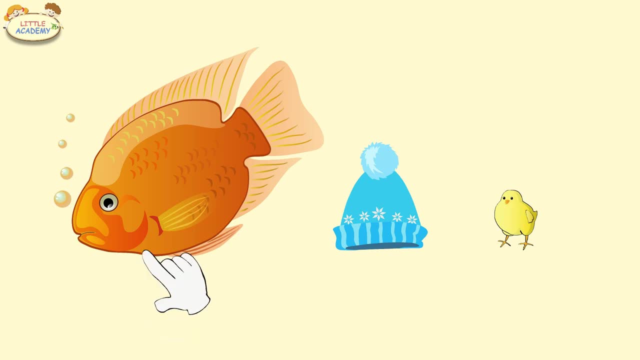 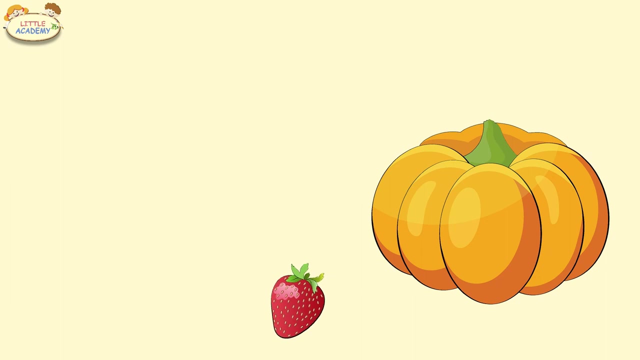 Now tell me What's the size of this fish. That's right, the fish is large. And what size is the hat? Yes, the hat is medium size. What about the chick? Great, the chick is small. Let's take a look. 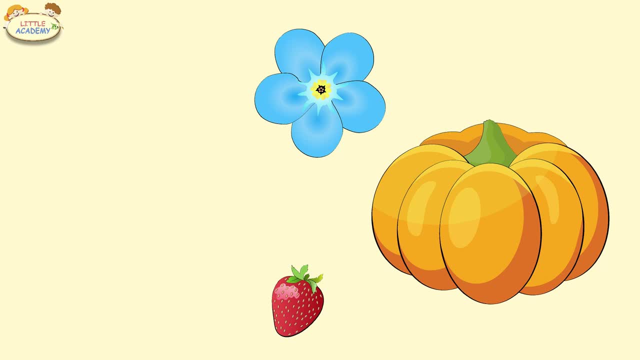 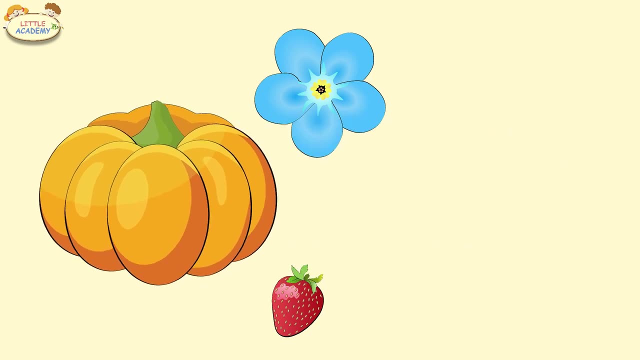 Here are three objects: A pumpkin, a flower and a strawberry. Which is the large one? Great, it's the pumpkin. Which one is the big one? The pumpkin, Which one is medium? Yes, the flower is medium, And which one is small? 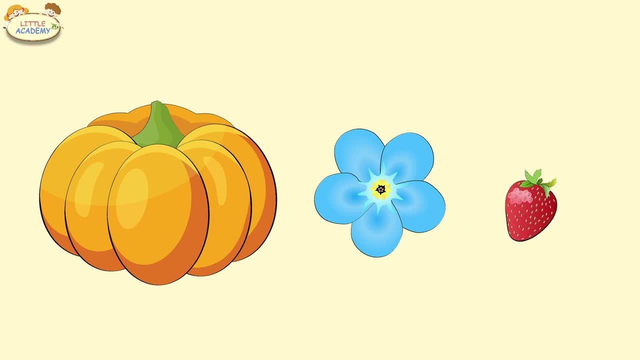 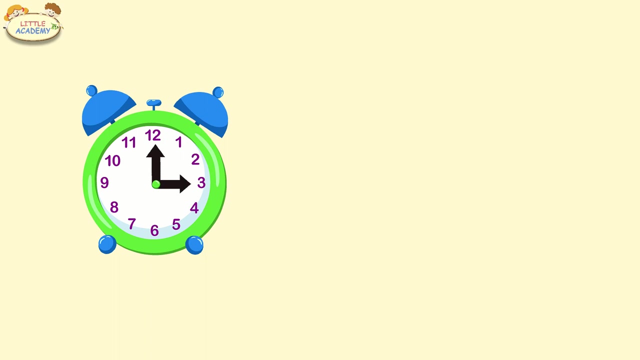 That's right, the strawberry is small. Great job, Now you know how objects can be different sizes. Now let's see how we can compare the objects. This alarm clock is large, This one is smaller, This one is even smaller And this one is the smallest. 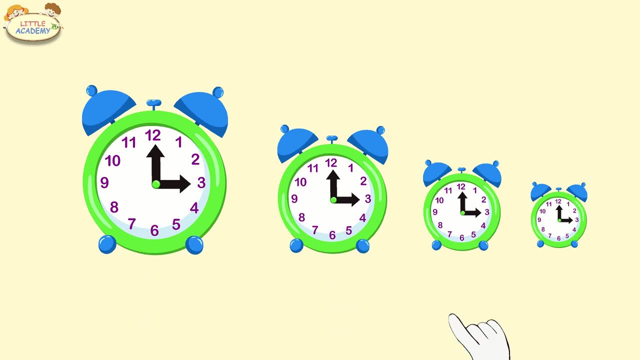 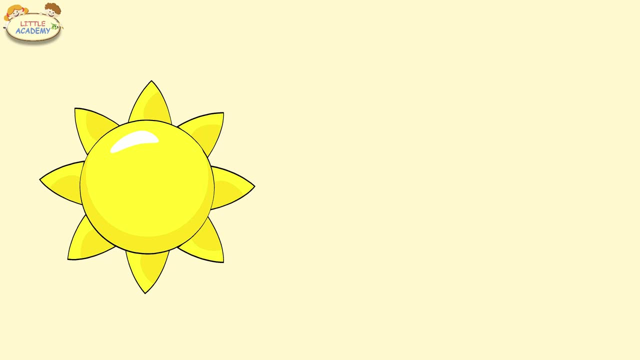 Large, smaller, even smaller and the smallest. Look again: The sun is large, The fir tree is smaller, The plum is even smaller And the shell is the smallest. So this object is the largest, This one is smaller, This one is even smaller. 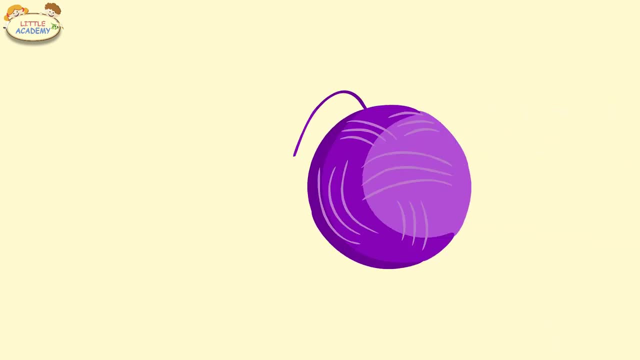 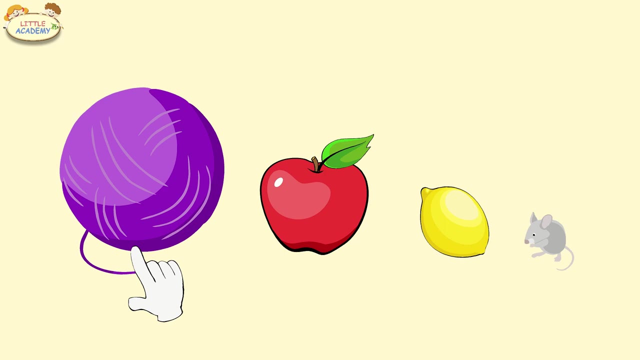 And this object is the smallest. Now tell me what size is the ball of yarn. Good job, The ball of yarn is large. What about the apple? The apple is smaller. What about the lemon? Yes, the lemon is even smaller. 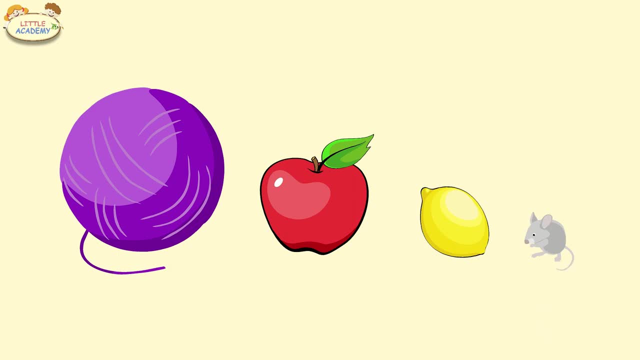 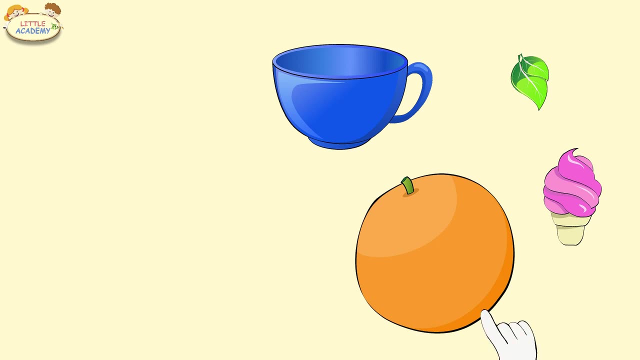 And the mouse. The mouse is the smallest. The apple is the smallest. Yes, the apple is the smallest. Let's see which of these objects is the largest. That's right, The orange is the largest. Which object is smaller? Yes, the cup is smaller. 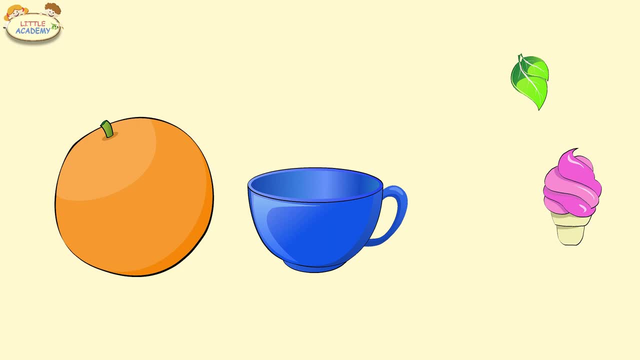 Which object is even smaller? The ice cream is even smaller, The ice cream is even smaller. And which one is the smallest? Yes, the leaf is the smallest, But But Great job. Now let's compare the objects a little differently. 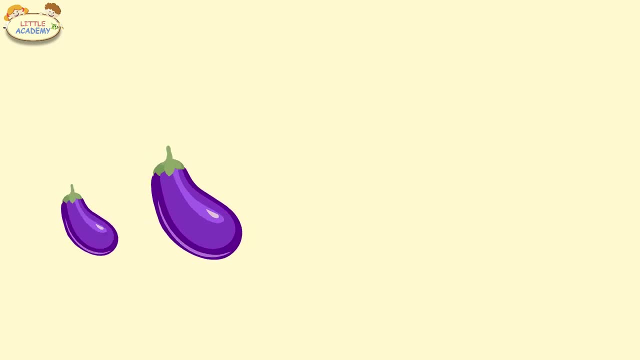 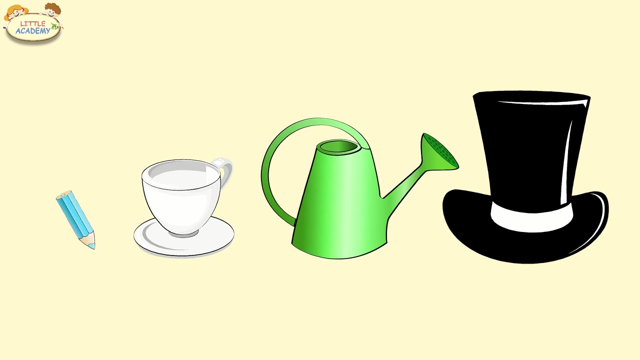 This eggplant is small, this one is larger, this one is even larger and this one is the largest: Small, larger, even larger and the largest. Let's do it again. The pencil is small, the cup is larger, the watering can is even larger, the top hat is the largest. 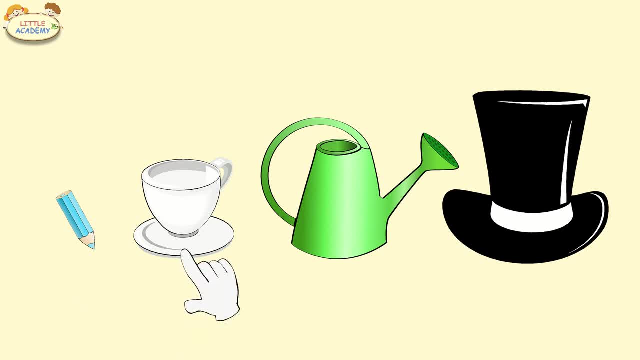 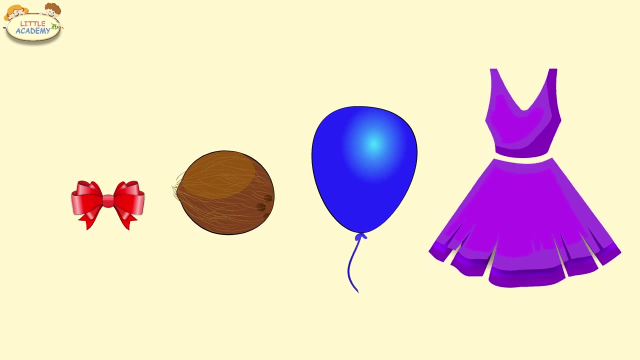 This object is small, this one is larger, this one is even larger and this one is the largest. Now tell me What is the size. What is the size of the bow? Good job, The bow is small. What about the coconut? 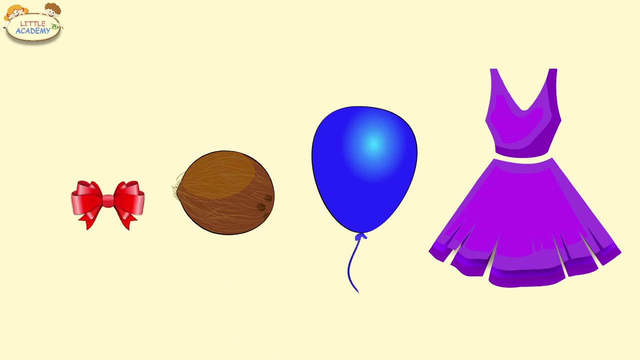 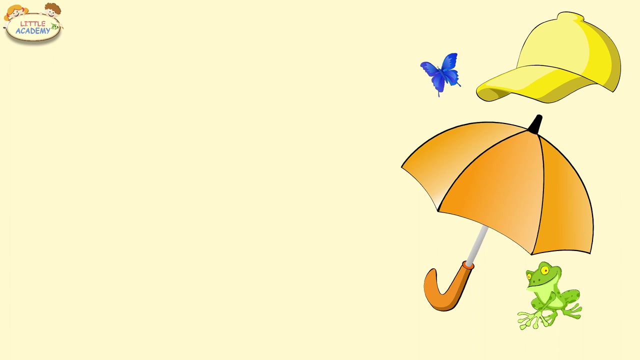 That's right, the coconut is larger. What about the balloon? Yes, the balloon is even larger. And the dress? The dress is the largest. Very good, Now let's see which of these objects is the smallest. Yes, the butterfly is the smallest. 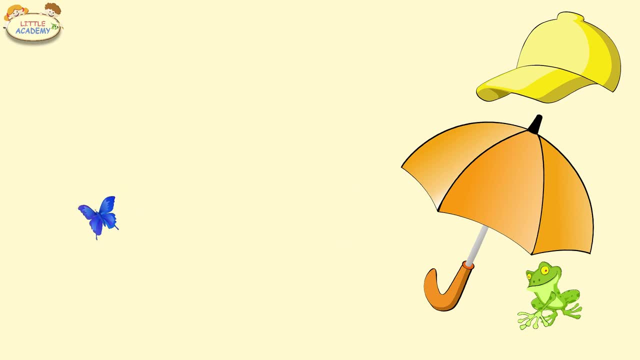 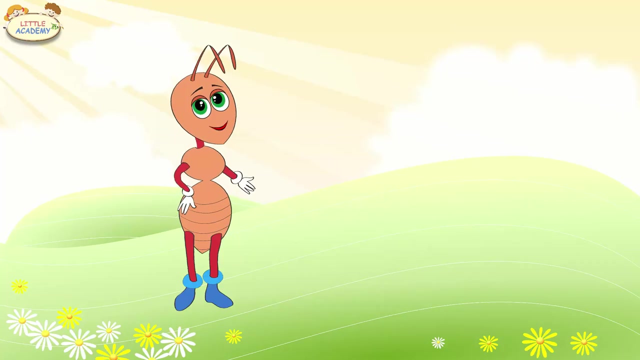 Which object is larger? The frog is larger. What is even larger? Correct, the cap is even larger. And what is the largest? Great, The umbrella is the largest. Awesome. Now I will tell you how objects can be the same, similar and similar. 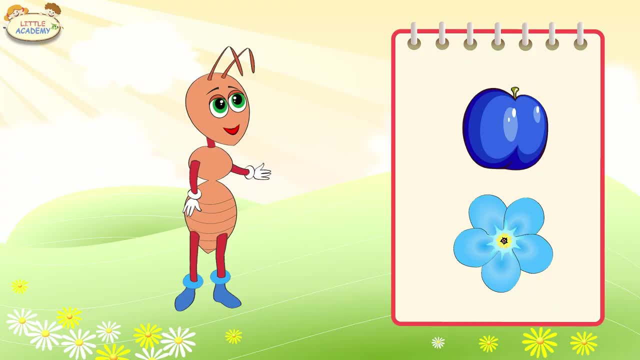 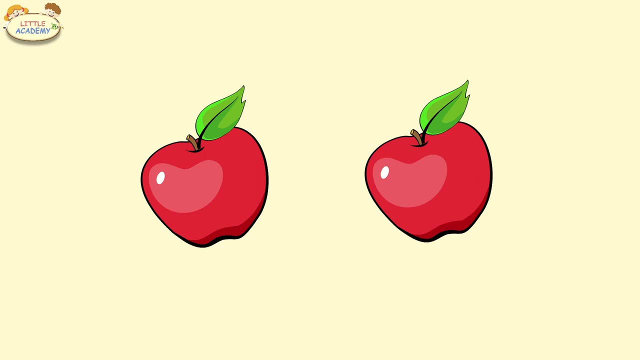 Let's see. Here are red apples. They are the same. Here are more apples: red and yellow, They are similar. And here is an apple and a fir tree. These objects are different. Let's do it again. Here are blue vases. 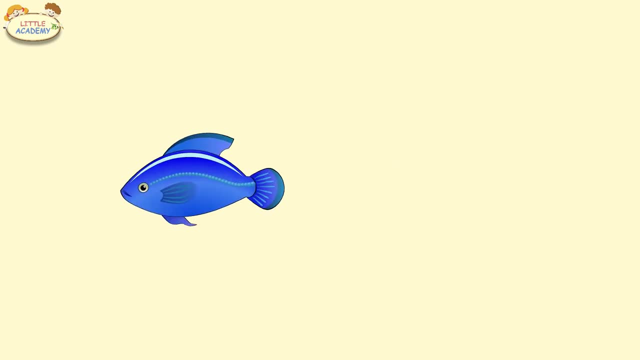 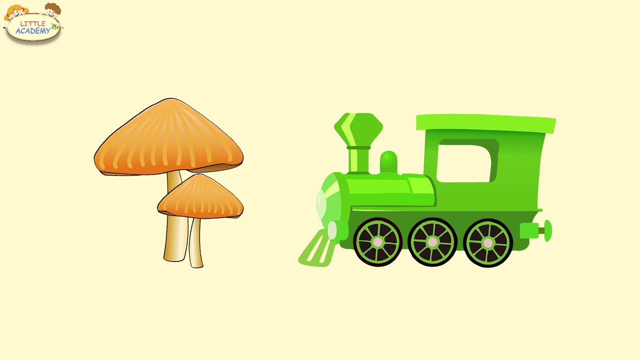 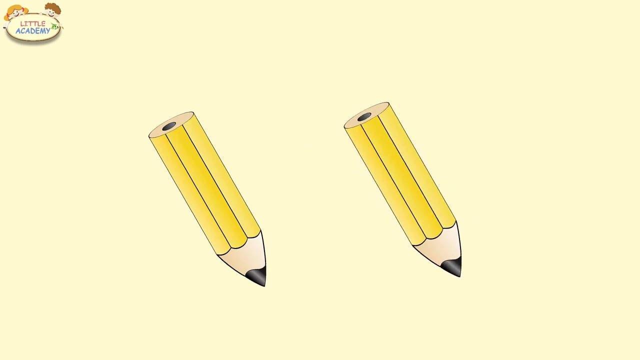 They are the same. Here are fish. They are similar, And here are mushrooms and a train. These objects are different. Now look, Are these objects the same, similar or different? That's right, These pencils are the same. What about these objects? 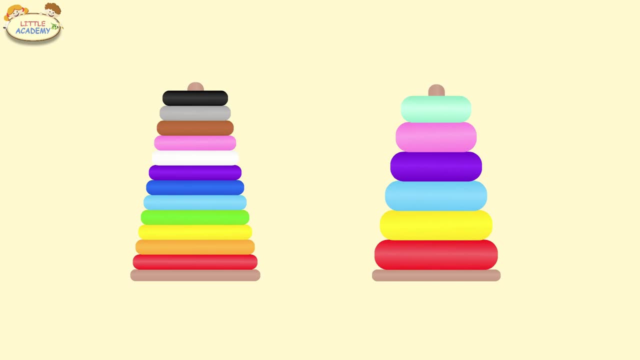 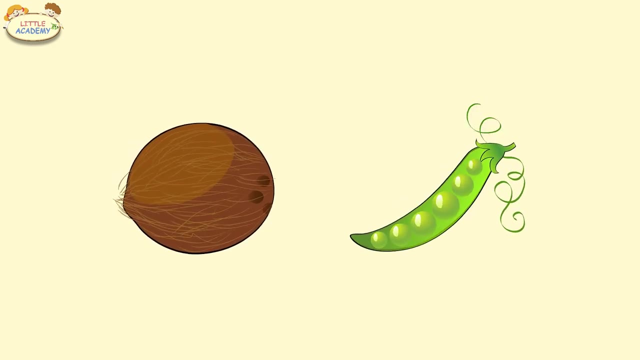 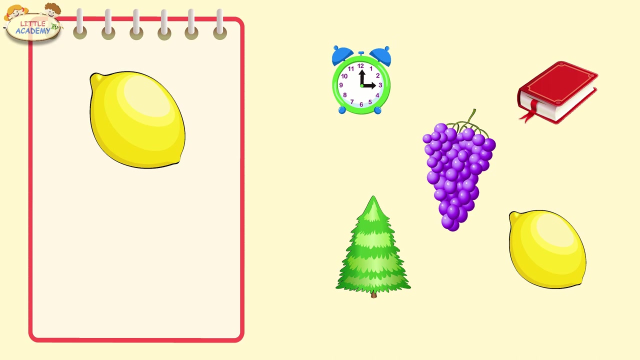 Are they the same, similar or different? Yes, these stackers are similar. Now take a look at these objects. Are they the same, similar or different? Yes, of course they are different. Here is a lemon. Now let's look at these objects and find the same one. 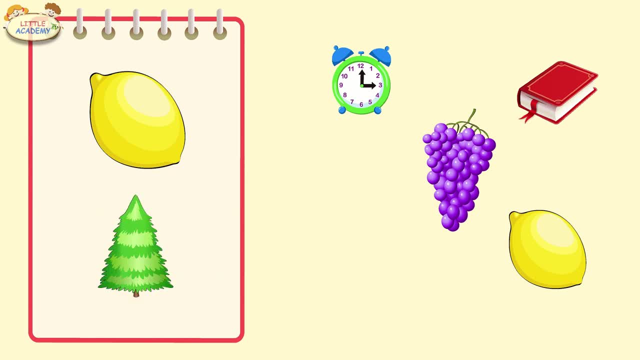 Is this one the same? No, this object is different. Maybe this one is the same. No, this one is also different. Maybe this one. No, it's different. Is this one the same? No, it's not. Then maybe this one. 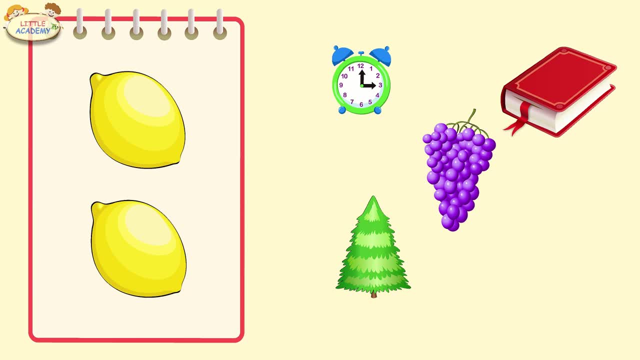 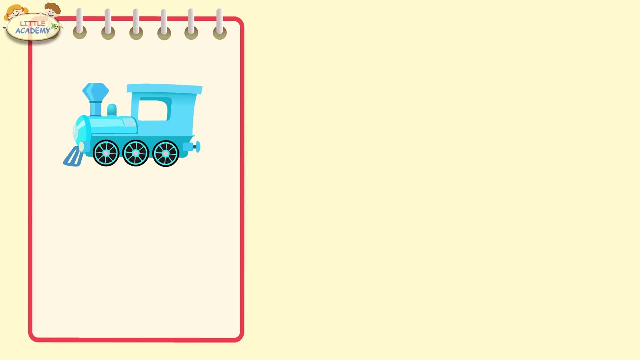 Yes, these lemons are the same. Here is a train. Let's look at these objects and find one that's similar. Is this one similar? No, these objects are different. Is this one similar? No, these objects are also different. 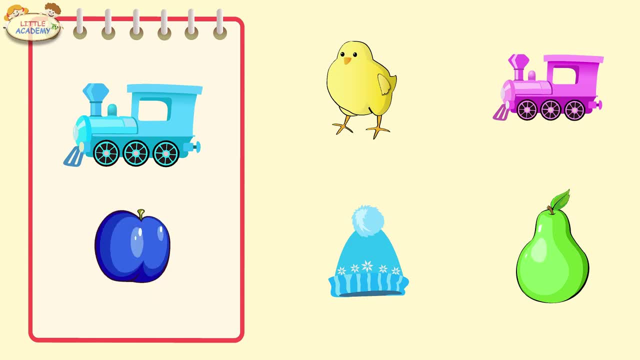 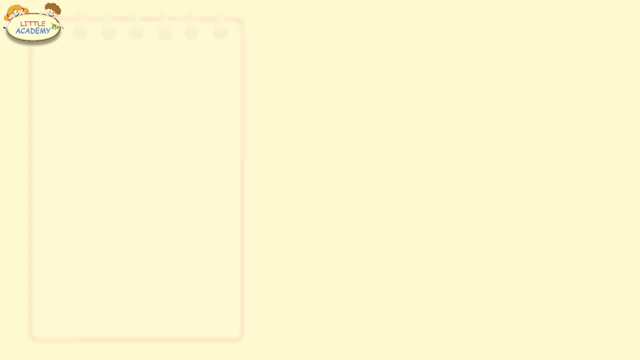 Maybe this one is similar. No, this one is also different. Maybe this one? No, it's different. Then maybe this one? Yes, that's correct, These trains are similar. Here is a mouse. Let's look at these objects and find one that's different.